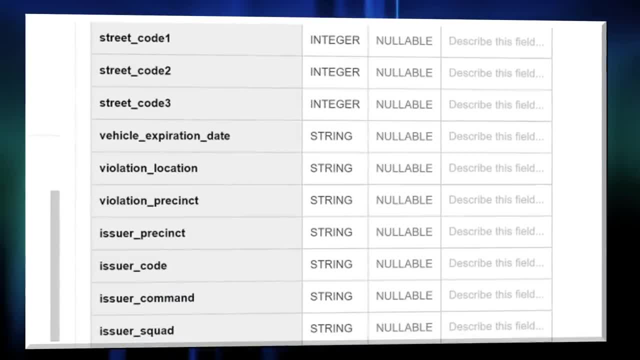 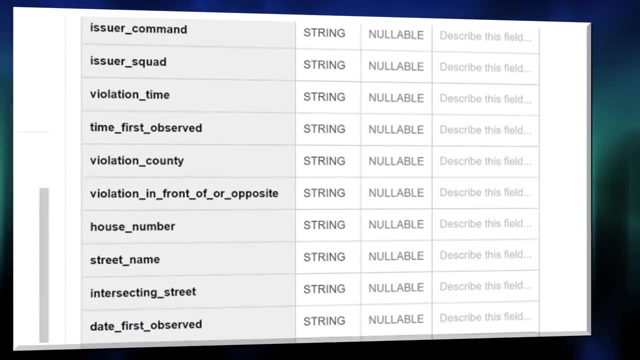 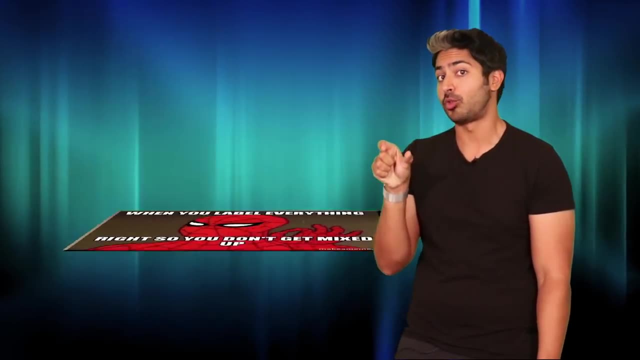 or too complicated to understand. But AI wizards are delighted because we know that there's so much we can do. We can create and discover with the data set using machine learning. Hopefully, the data set is labeled. This is a column that describes what each data point is. Think of it as a summary of what 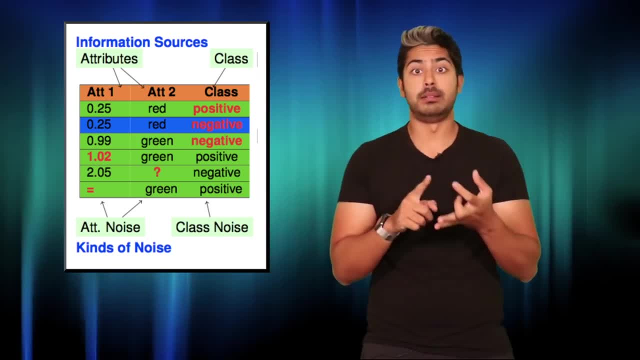 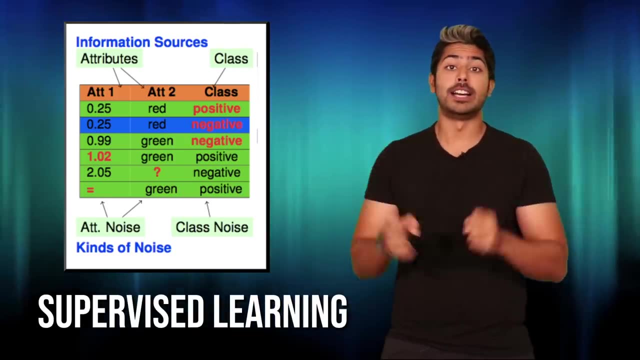 all those signals mean This could be a dog, an emotion, a diagnosis, an adolescent phase, so many things. We can then consider this a supervised learning task, And if it doesn't have labels, then it would be considered an unsupervised one. 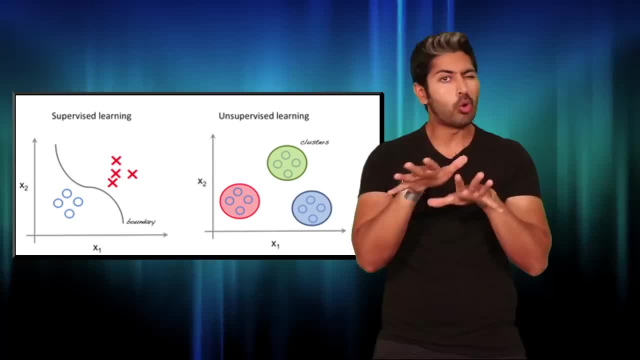 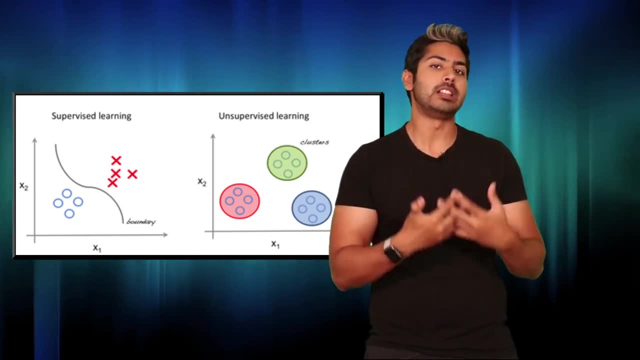 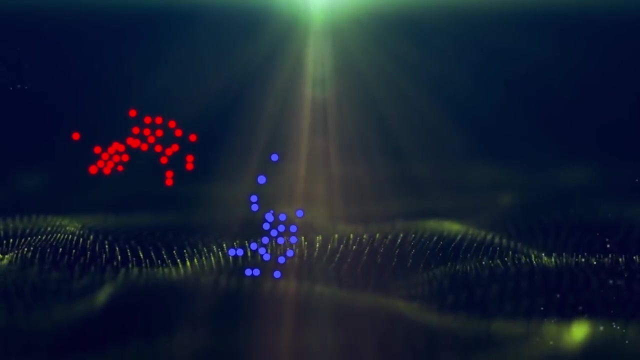 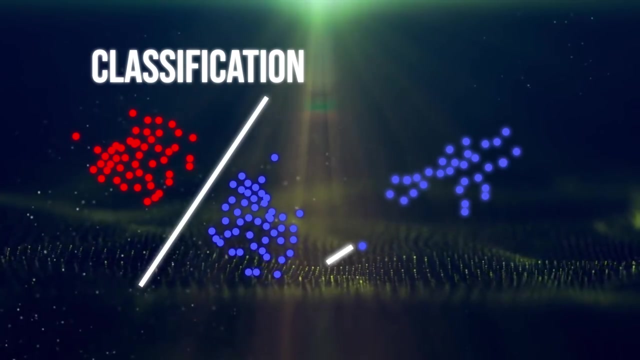 This is more of an exploratory problem, where we don't have a target label we're trying to predict. Instead, we use mainly clustering techniques to make discoveries. Supervised learning can be broken down into two types of problems: regression and classification. Regression is when we want to predict an output value that can have a lot of different values. 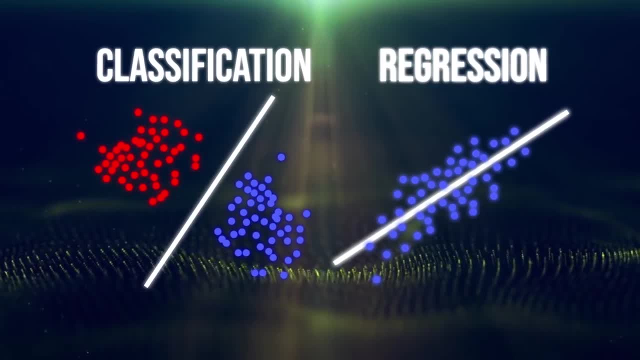 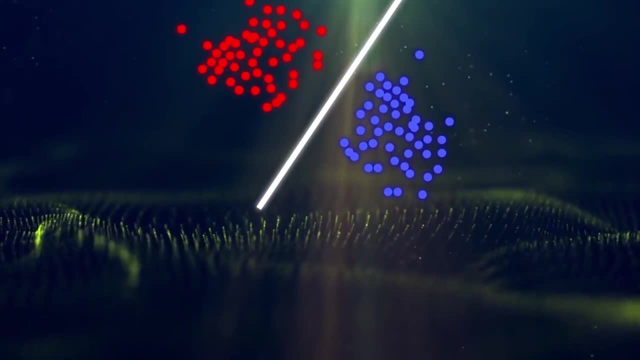 And usually our output is some rapid, linear or random type of output. Classification is when we want to predict an output that can only have some specific categories. Now, depending on the type of problem we have, we can choose a suitable algorithm to. 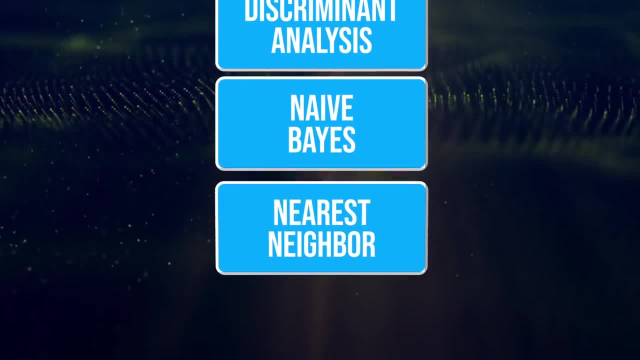 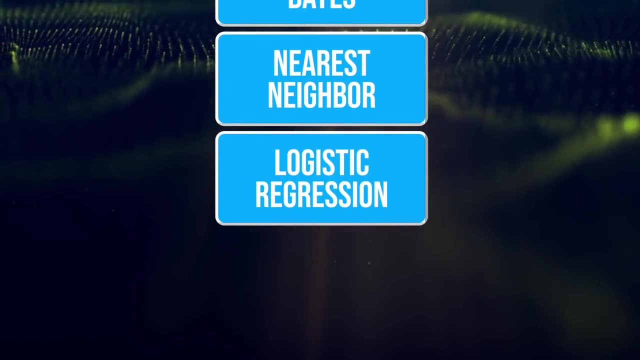 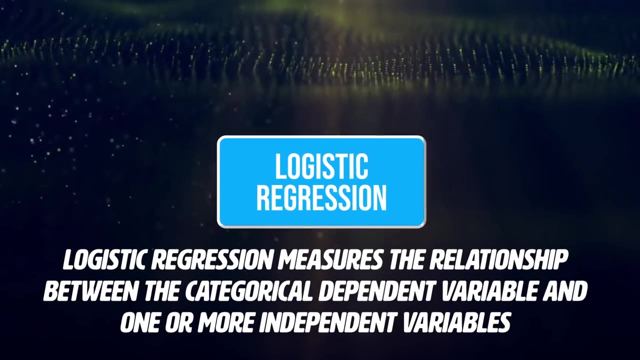 solve it. One algorithm that is frequently used to solve supervised classification problems is called logistic regression. It measures the likelihood occurrence of an event. Logistic regression measures the likelihood occurrence of an event. So some possible questions that logistic regression could answer include: how likely is it that a user will purchase? 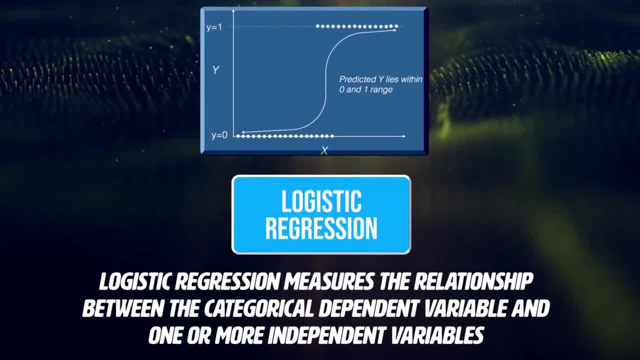 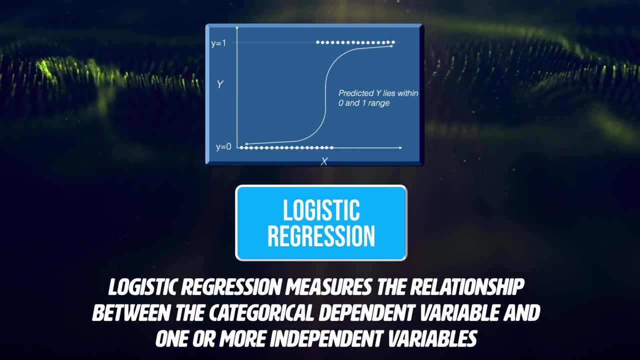 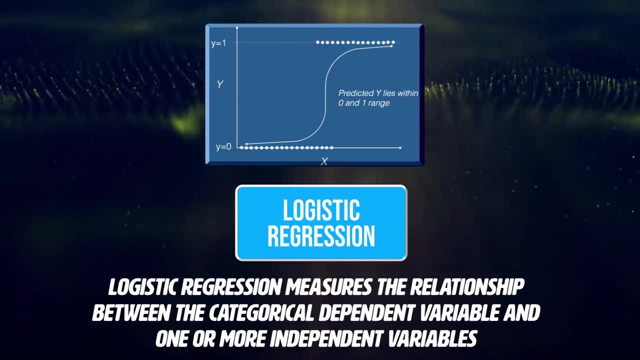 a subscription. How likely is it that France will win the world cup? How likely is it that getting a certain test score will result in admission to a good university? How likely is it that a tweet from Kanye makes sense Once our model outputs a class likelihood percentage for a new data point? 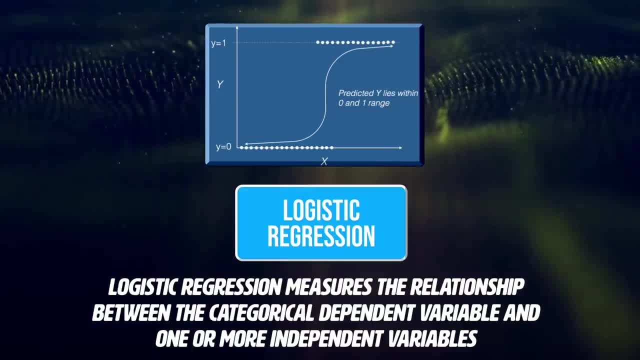 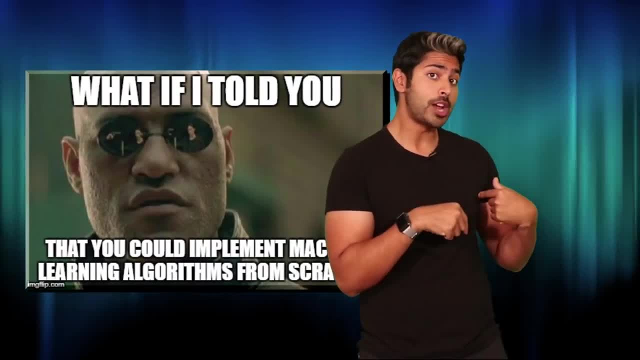 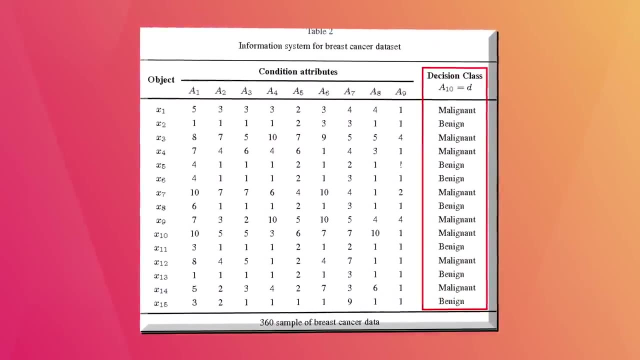 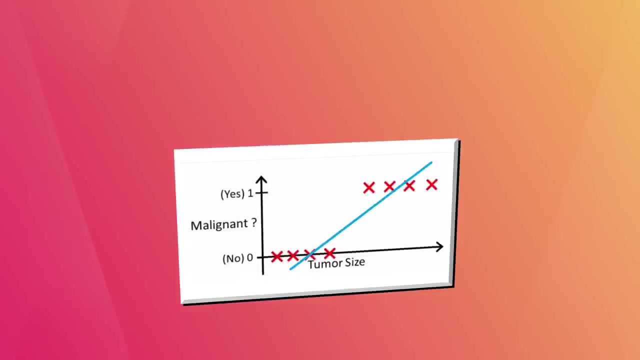 we can then use that to classify that data point accordingly. You might be wondering why we use logistic regression and not linear regression for this. Well, suppose we had a labeled dataset of cancerous tumor sizes. Each was either malignant or not, denoted by either a 0 or 1.. If we used linear regression we'd construct the line of: 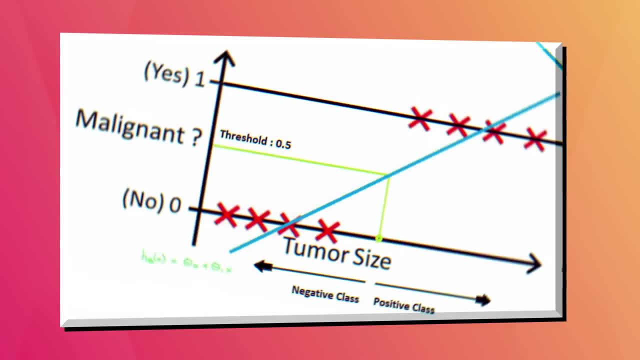 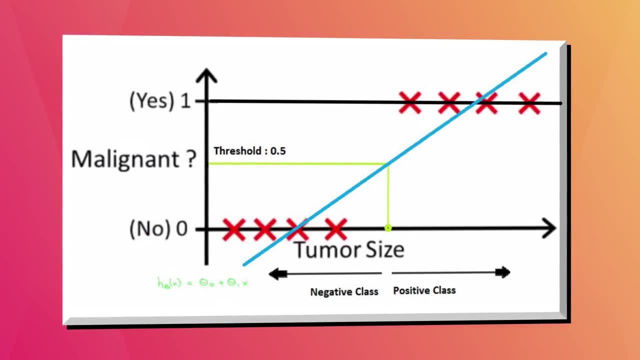 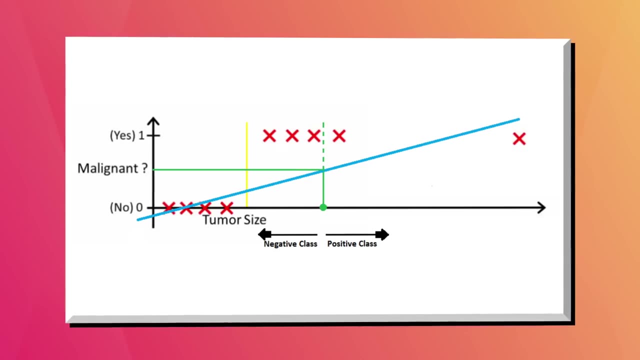 best fit for the data and graph it. We could then decide that all the values to the left of the line are considered not malignant and all the values on the right as malignant. But what if there's an outlier in the data, A data point that is significantly different? 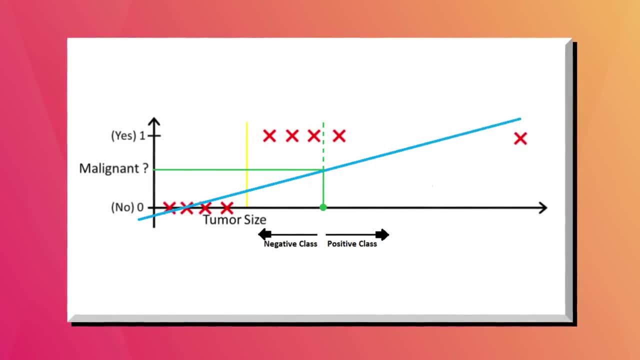 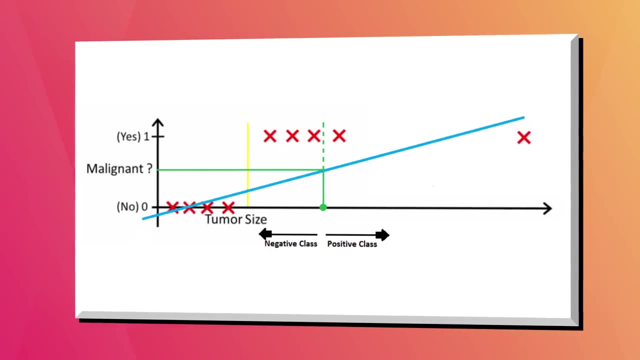 than the rest. If we accounted for that outlier point when we built our linear regression line, it would look pretty warped. It'll put some positive class examples into the negative class. If we were to draw out an imaginary class decision boundary that divides malignant tumors from benign tumors, it would look off. It should have been in a different spot. 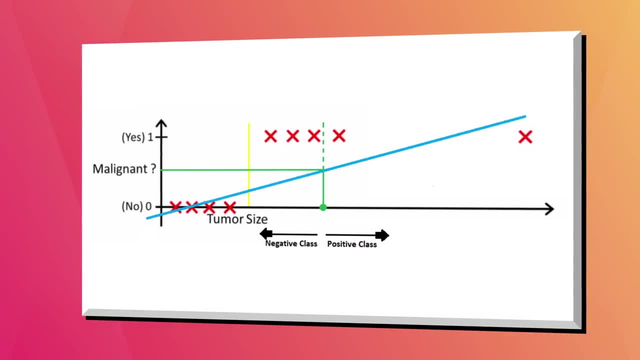 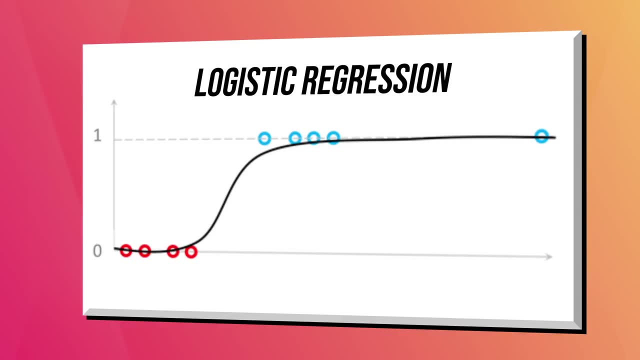 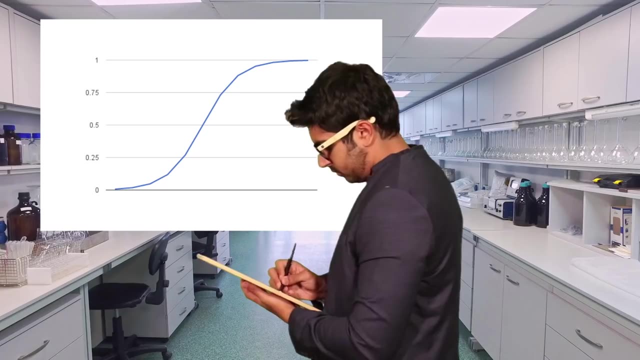 but a single outlier threw off our linear regression predictions. We need a way to deal with outliers in the data. Logistic regression helps us do just that because it uses the standard logistic function. This was developed by statisticians to describe properties of population growth in ecology. 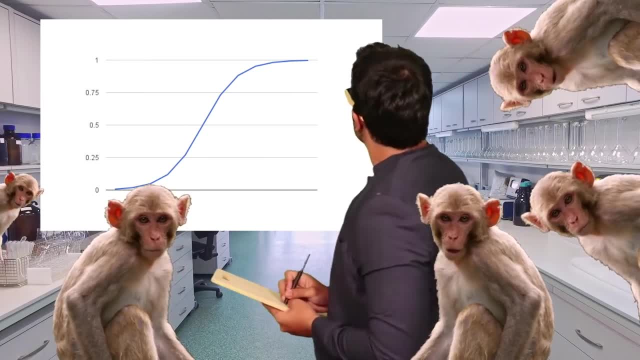 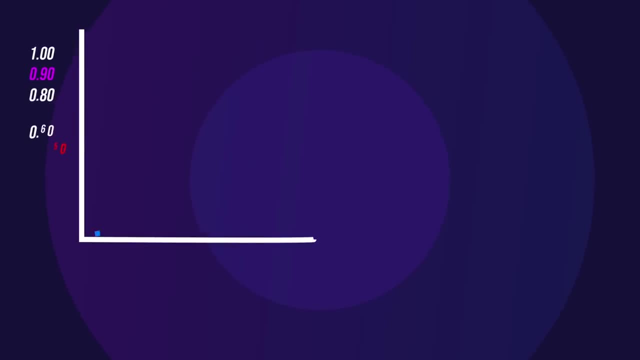 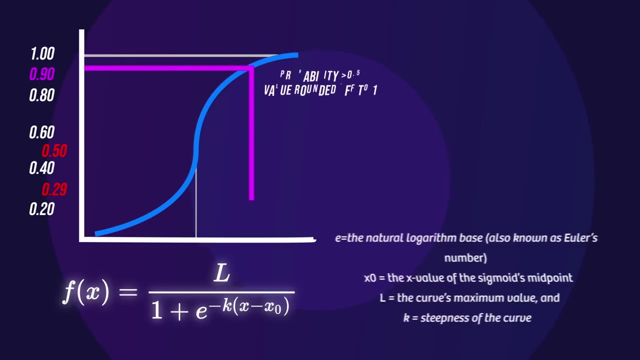 rising fast and maxing out at the carrying capacity of the host environment. It looks like an S-shaped curve that takes any real number and maps it into a value between 0 and 1, but never exactly those limits. This is described using the equation F of X equals L over. 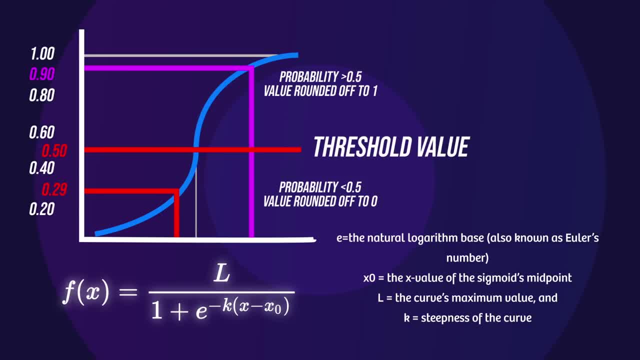 1 plus e to the negative k times the difference between x and the x-value of the curve's midpoint. L is the curve's max value. So if we were to draw a graph that looked like this, it would say that the curve's midpoint is the curve's max value. 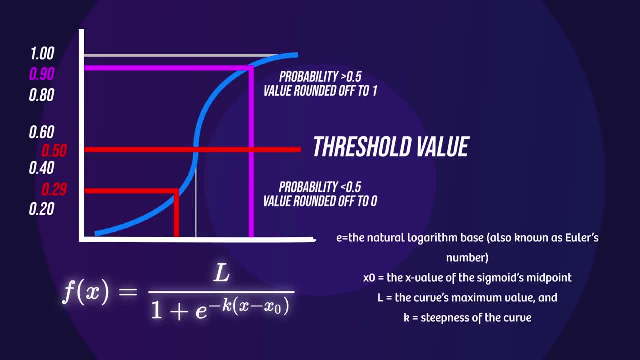 E is the natural logarithm base, a constant value used throughout math to help model growth, And K is the steepness of the curve. Logistic regression actually uses a special case of the logistic function called the sigmoid function. This is when L equals 1, because it's using binary classification values for its prediction. 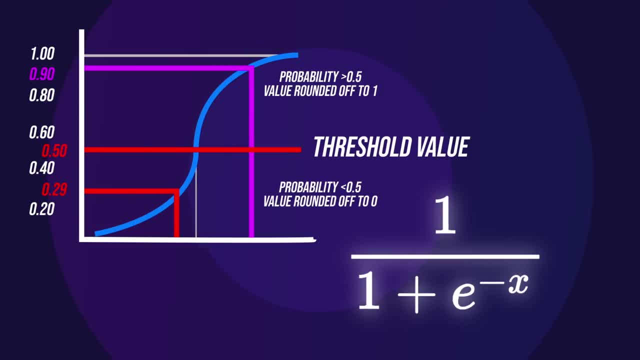 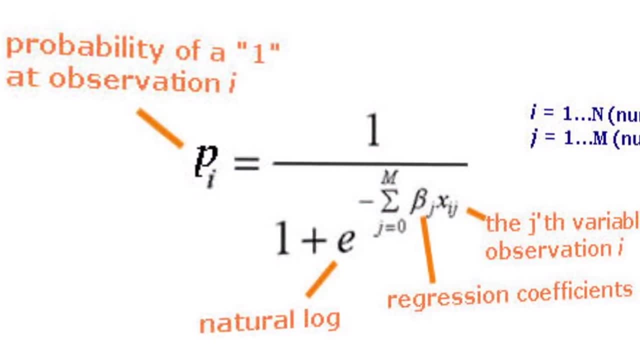 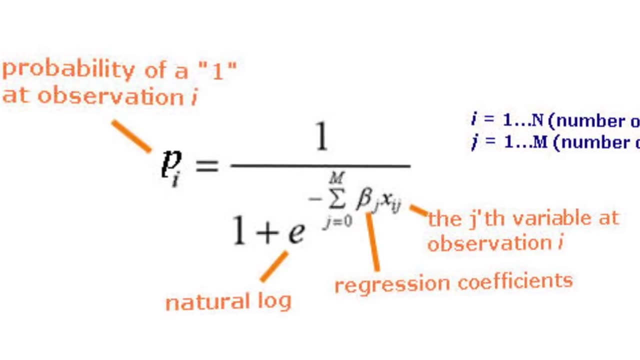 either 0 or 1.. And K will be set to 1 as well, making a simpler equation. What logistic regression does is it uses a linear function to represent the input values. That's where the input values are combined linearly using weights or coefficient values. 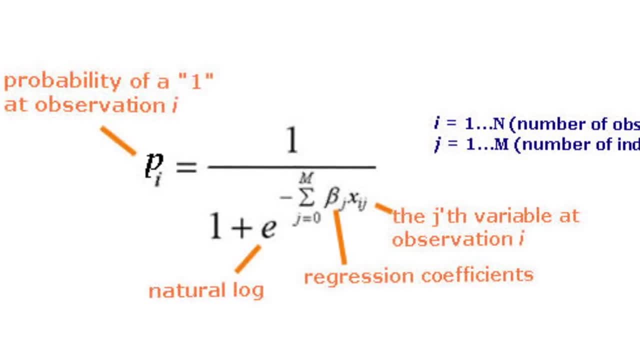 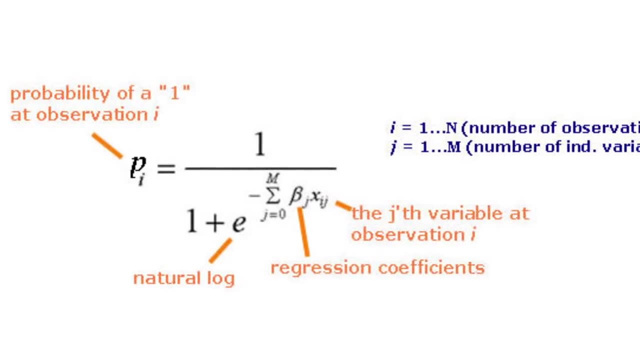 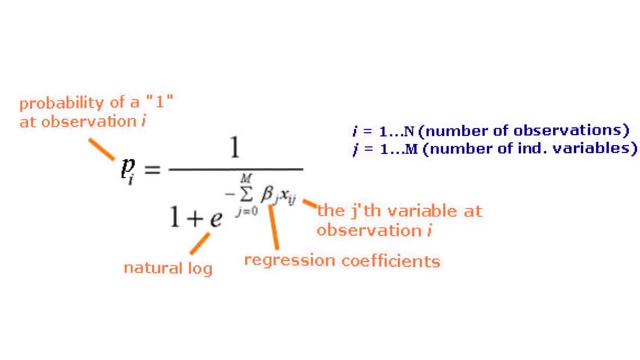 often referred to as the Greek capital letter, Theta- to predict an output value y, Thanks Greece. The difference from linear regression, though, is that the output value being modeled is a binary value- 0 or 1, rather than a numeric value. We do this by plugging that equation into our sigmoid function, which gives us the full. 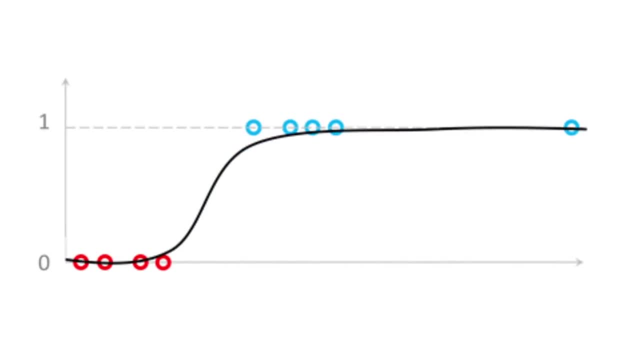 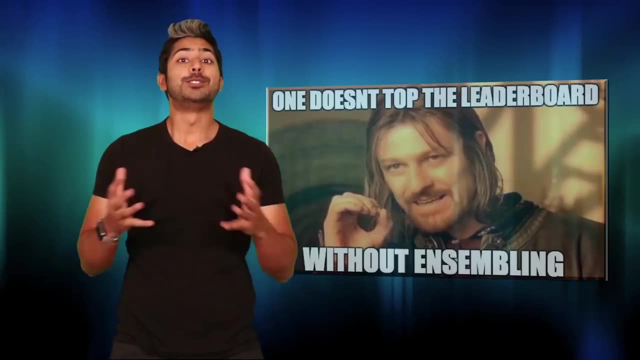 logistic regression equation. When we use this model instead of linear regression for our tumor dataset, it'll incorporate any outliers into it, So let's start building our app, shall we? It's a collection of labeled tweets that we can find on Kaggle. 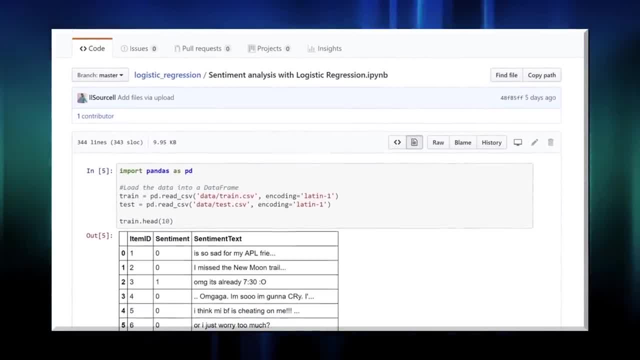 It's got both training and testing CSV files attached, so once we download the dataset, we can view it ourselves in our Kaggle app. So let's get started. So let's get started. I'm going to upload this image to my Jupyter notebook. 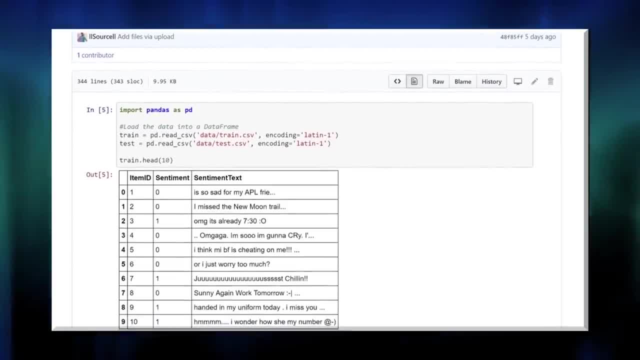 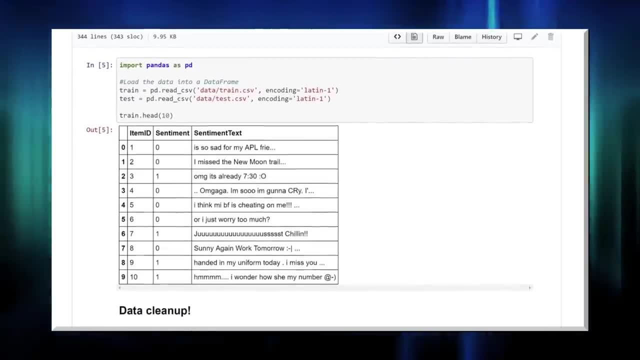 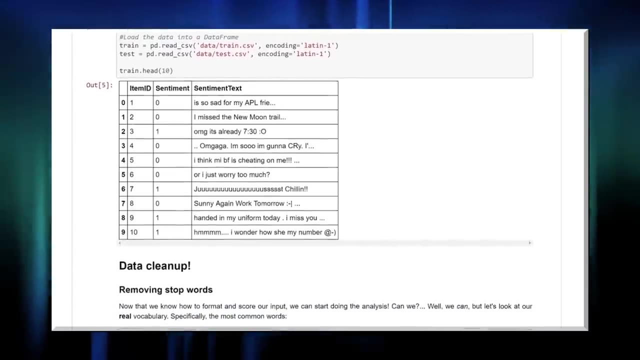 Once we spin it up, we can import the data pre-processing tool, Pandas, to help load the data into a modifiable data frame in memory Using the head function. we can see that the data contains three columns: The item, sentiment of the tweet- either 0 for negative or 1 for positive- and the tweet. 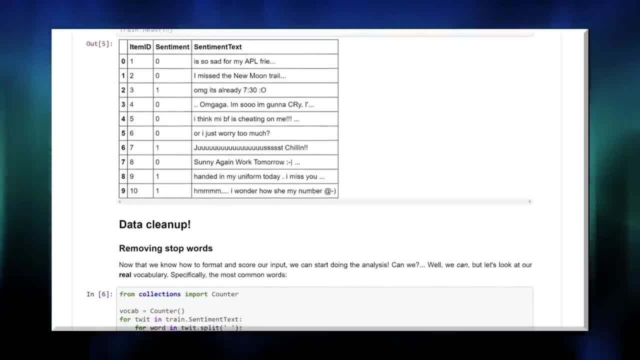 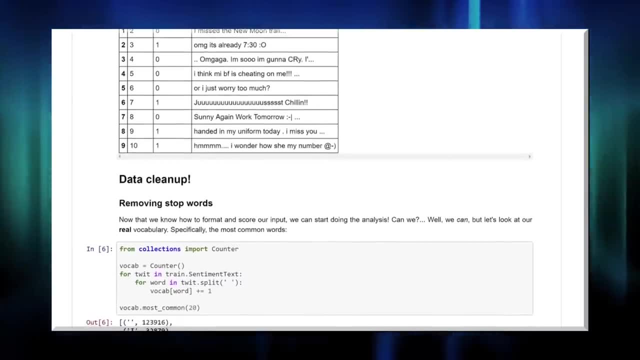 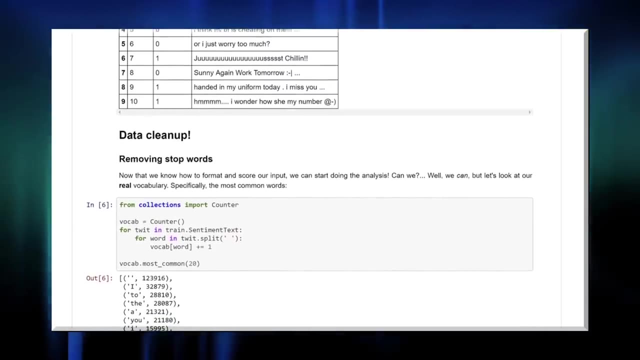 itself. Notice how these tweets are all different sizes. Some of them are much longer than the rest. An important data pre-processing step for us is to remove any unnecessary noise from our dataset. When it comes to text, there are a bunch of words that don't really contribute to the 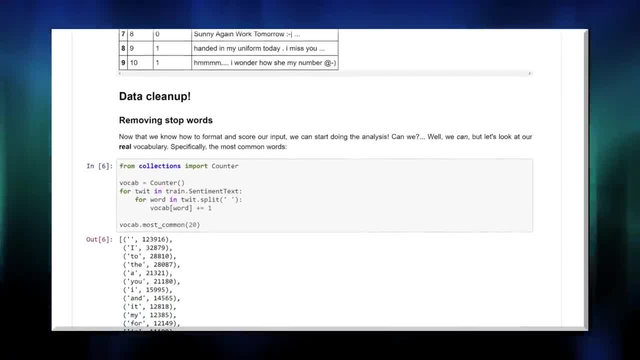 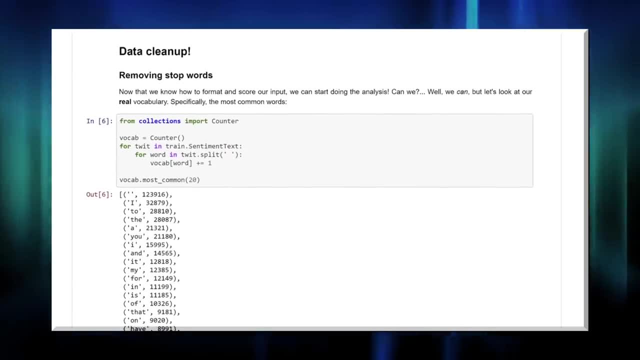 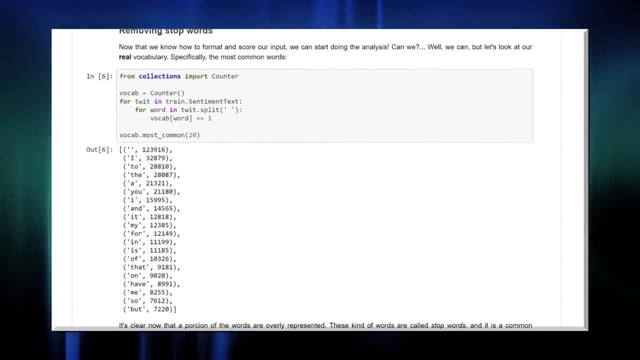 sentiment of the phrase as a whole. These are called stop words. Examples include the is, and of Using the NLTK library's stop word collection. we can iterate through the dataset and find any of the stop words that do exist and remove them. 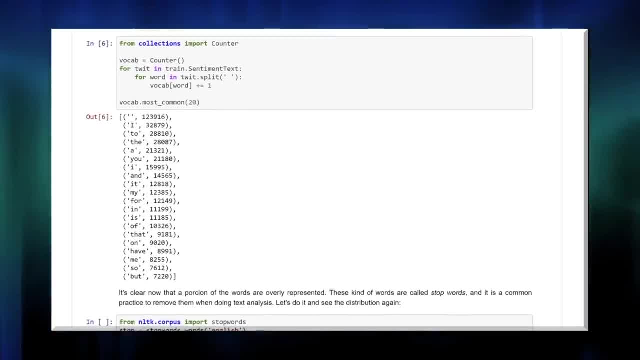 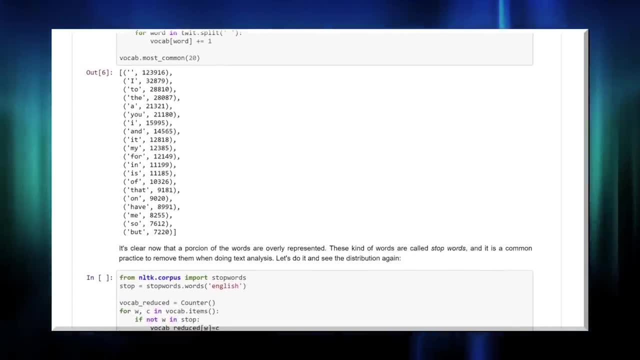 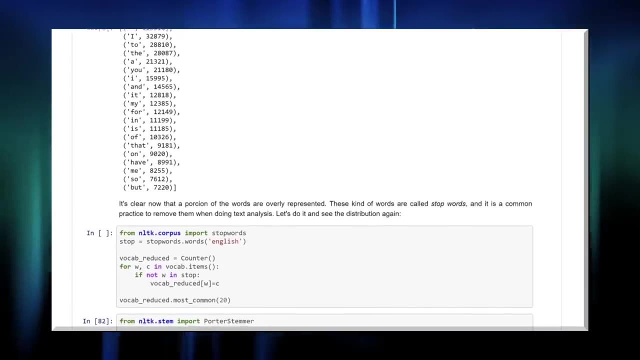 Once they're gone, we can go one step further in reducing noise by reducing our vocabulary size and consolidating similar words. For example, swag, swagger and swagalicious all have the same stem and we can just replace all of those instances with the stem swag. 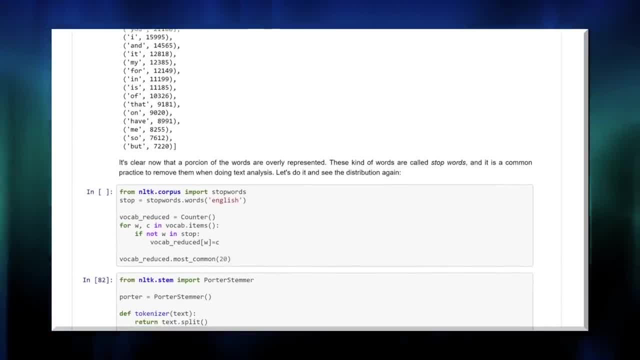 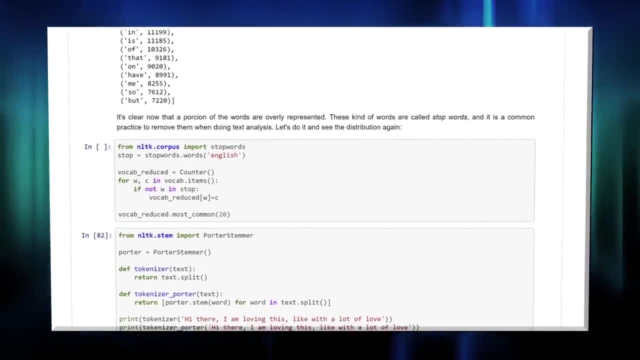 NLTK's got a handy stemmer module to help us do this automatically, And we'll also tokenize our words, meaning break each phrase down into individual words that form a larger vector. Train, train, train. I'm cleaning datasets, yeah. 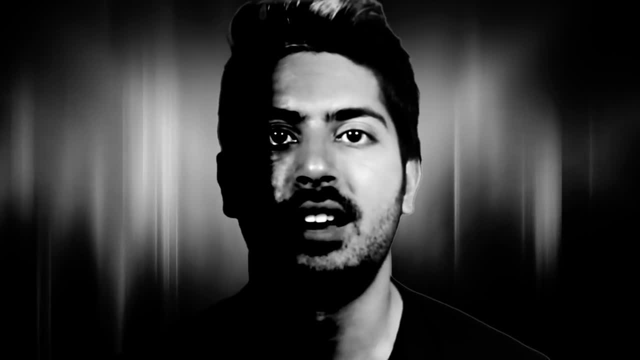 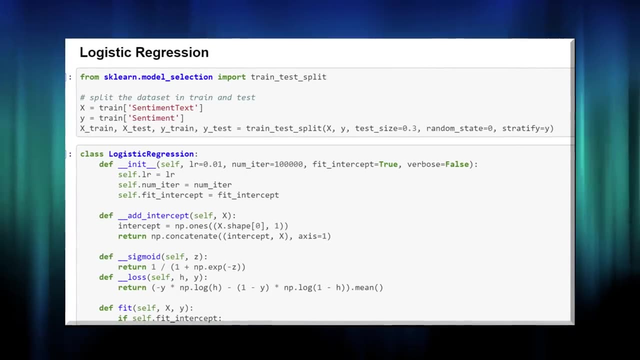 Trained it on my laptop. now it's on the internet. yeah, We can programmatically write out our own logistic regression class that we can use on the data later. It'll use two hyperparameters that we initialize when we call it. first, the learning rate. 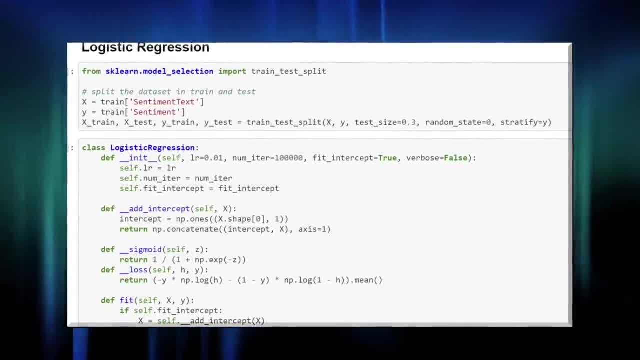 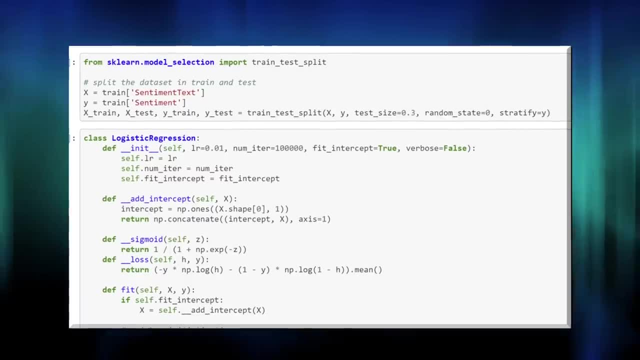 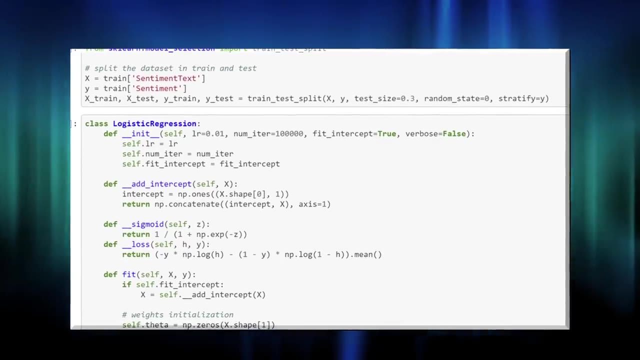 which controls how much we are adjusting the weights of our network during training. If it's too small, then optimization will be too slow, But if it's too large, our algorithm may fail to converge on the best result. Second, the number of training iterations we'll use. 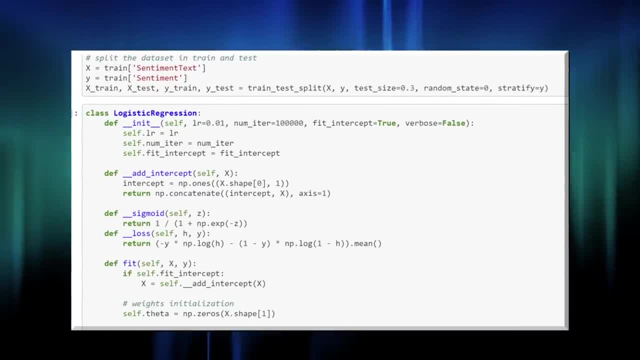 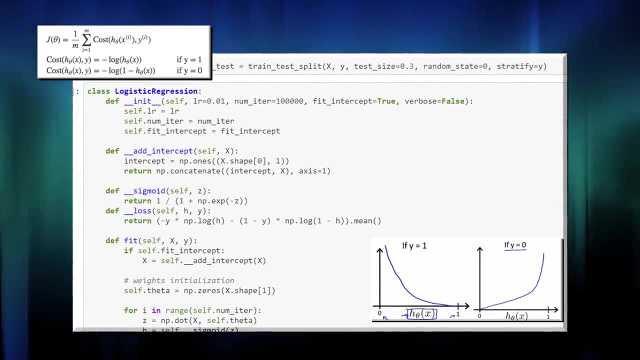 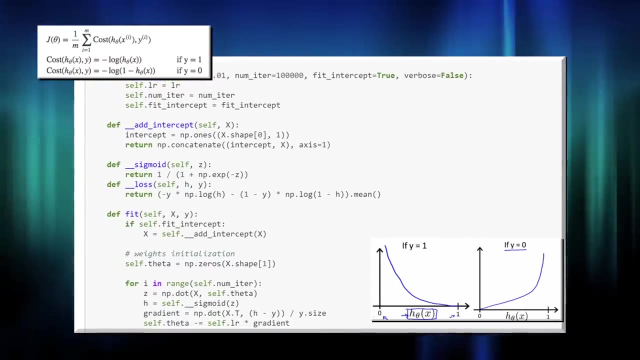 We can first write out the sigmoid function. since we already know the formula For our loss function, the way we measure how bad our prediction is compared to the real label, Let's use cross entropy. This can be divided into two separate loss functions, one of them for when x equals one. 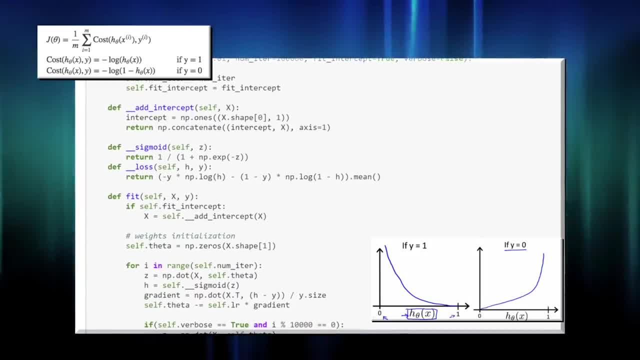 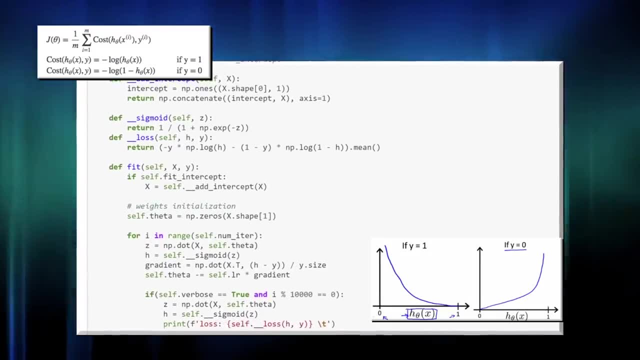 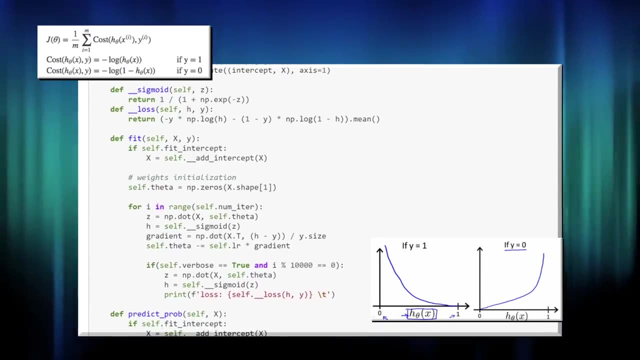 and one for when x equals zero. When we look at the loss function graphs for both of them, we can see the benefit of taking the logarithm. These smooth functions are always increasing or always decreasing and make it easy to calculate the gradient for our optimization process. 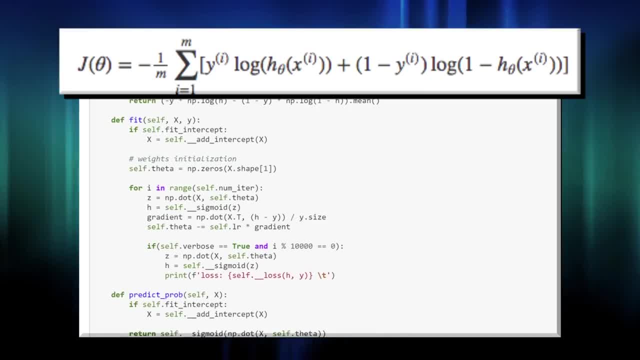 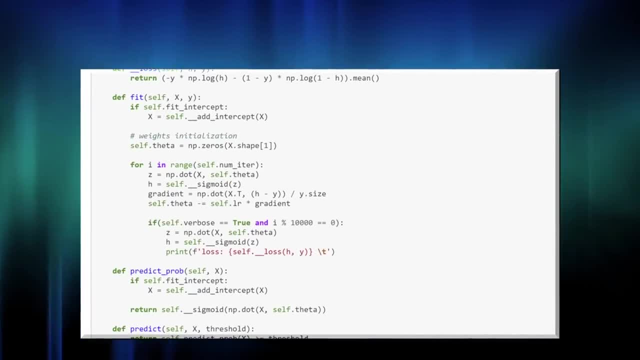 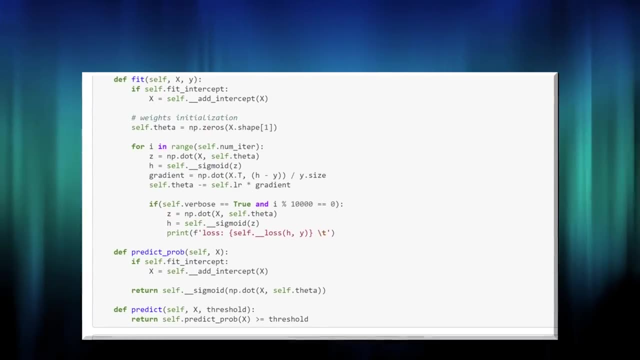 When we compress these functions into one, we get our final logarithm. Oh, and one more helper function before our training loop: add intercept. This will add a decision boundary to our graph. In our fit function we'll initialize the weights of our network as theta, then the 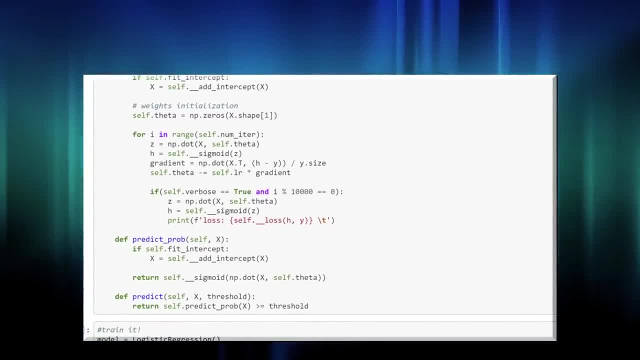 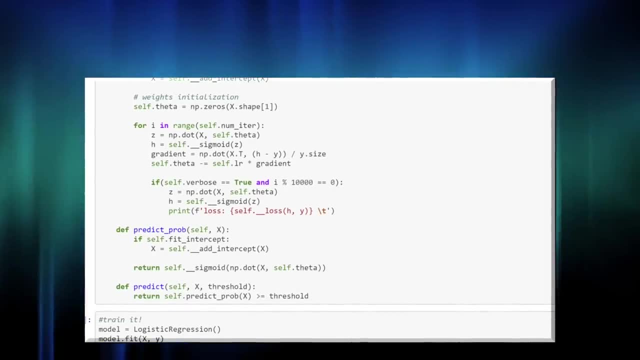 specified number of iterations. We'll compute the linear function by multiplying our input by our weight matrix, then use that as input to our sigmoid function to compute the output. We'll then compute the gradient by multiplying the transpose of our input to our output. 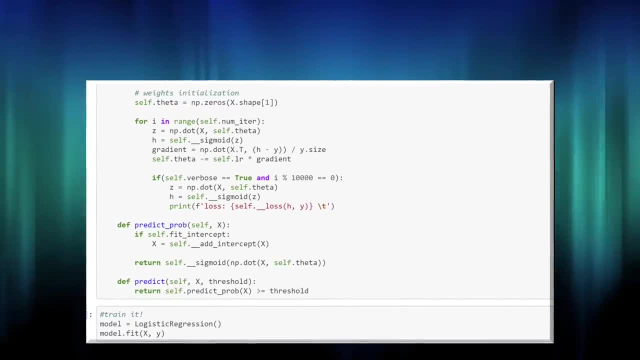 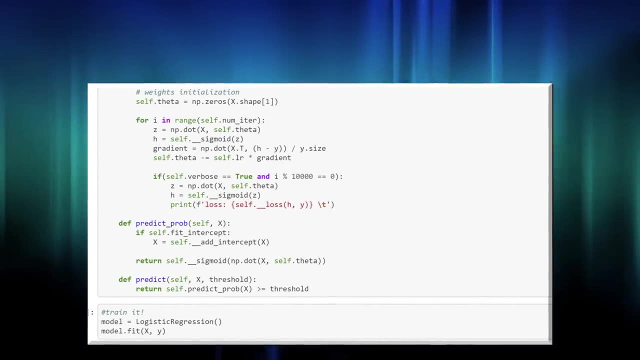 We'll then compute the gradient by multiplying the transpose of our input to our output data by the difference between our prediction and actual label. Once we multiply it by the learning rate, we'll adjust our weight value theta, to help make a better prediction next round.